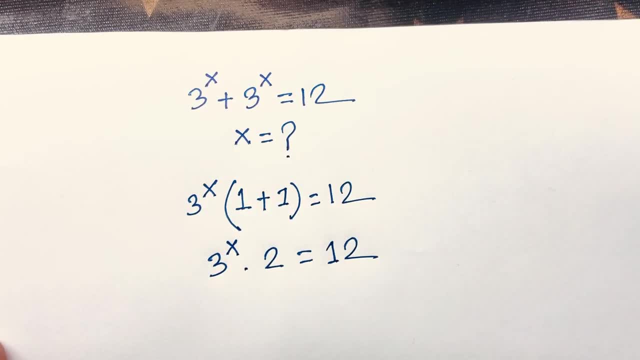 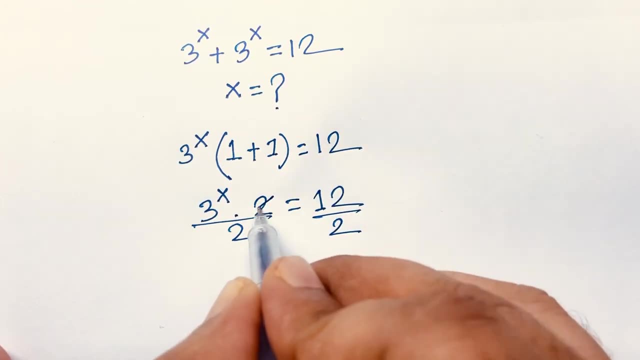 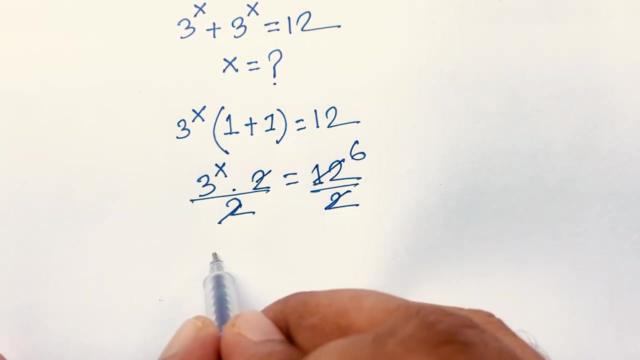 be 2 is equal to 12.. Then at this moment I divide both side, 2.. So I can see easily: here is 2, here is 2.. So 2 to cancel and 12 divide 2, it will be 6.. So I can see easily this equation becomes 3 to the. 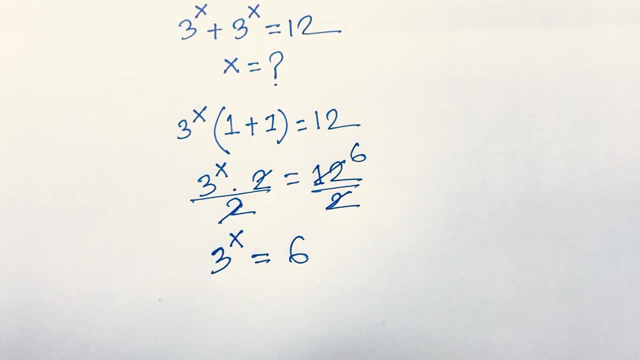 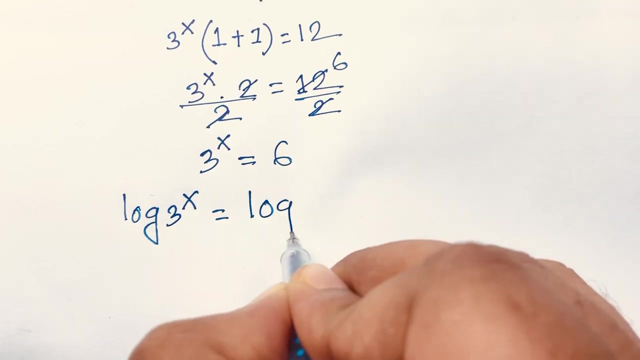 power x is equal to 6.. Yes, and at this moment, if I want to find out the value of x, So I use both side natural log So I can see easily. it will be: log 3 to the power x is equal to log 6.. Then, at this moment, according to: 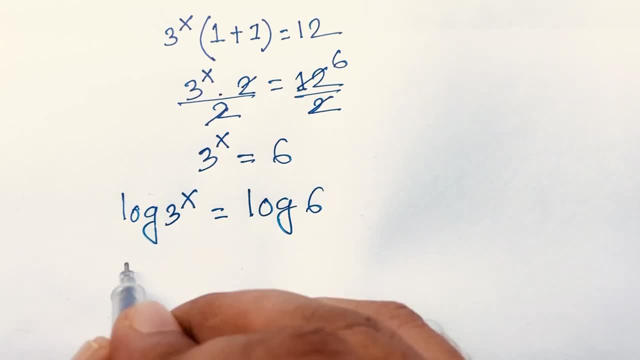 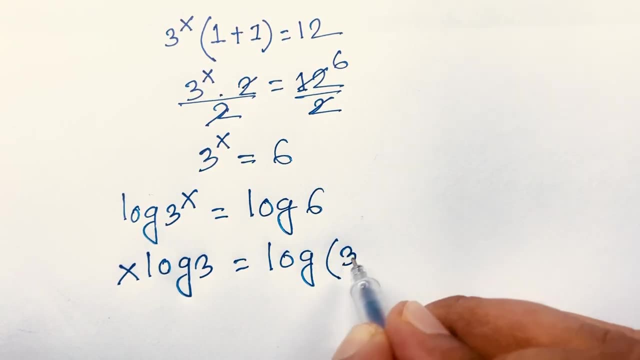 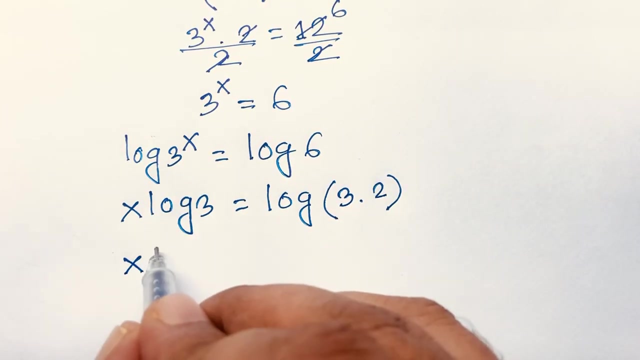 logarithm rules. I can see easily this x move on in front, So it will be x log 3 is equal to log 6. It will be 3 times 2. It will be 6.. Then I can see easily this equation becomes x log 3. and didn't know that log A V. 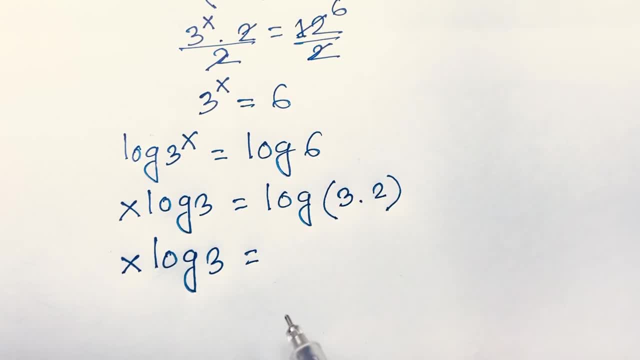 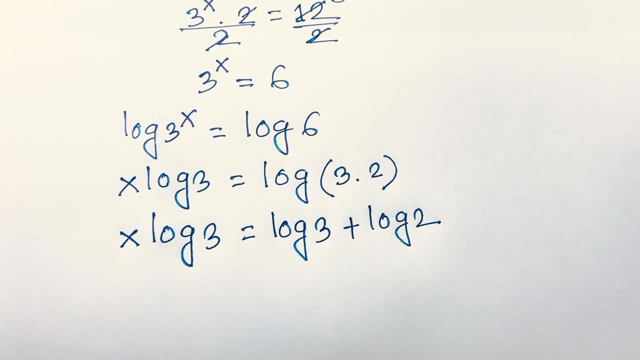 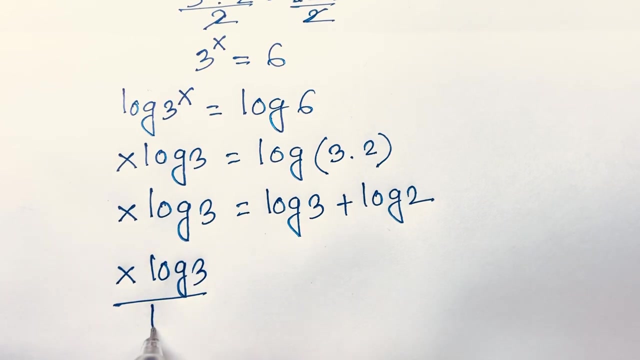 according to logarithm rules I can see easily- it will be log A plus log V. So log A plus log V, B is 2.. Then if I divide both sides, log 3. So I can say: x log 3 over 3 is equal to log 3 over log 3 plus log 2 over log 3. I divide both side, log 3. 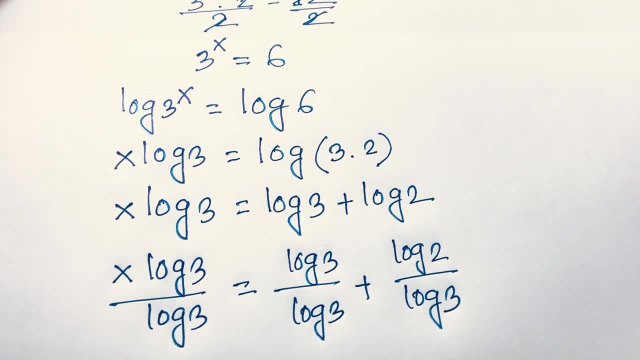 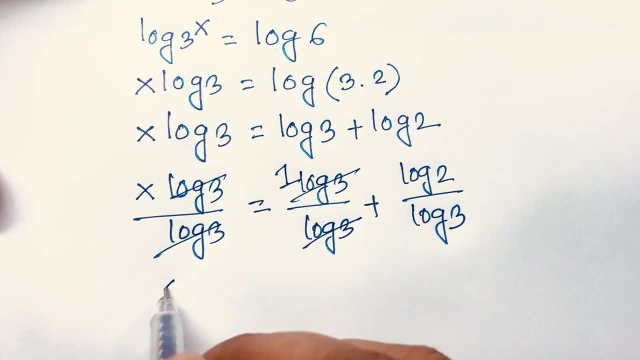 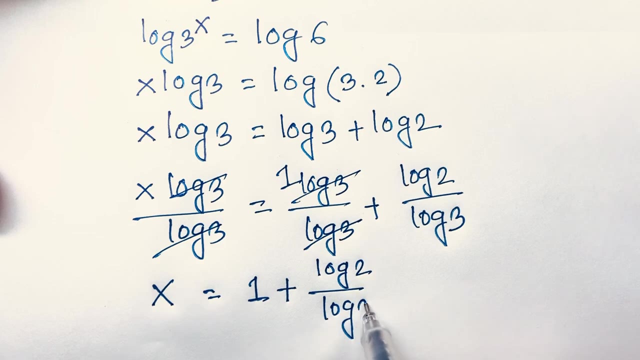 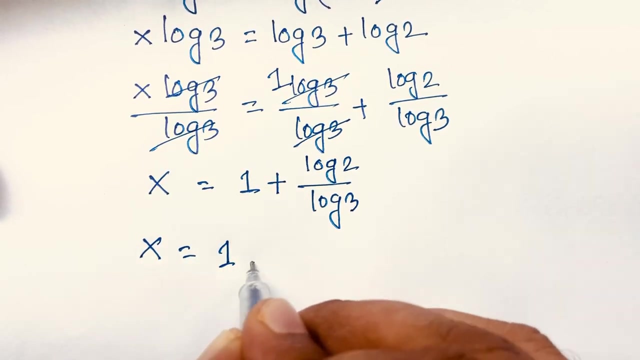 then I can easily: here is log 3, log 3 is cancelled. so this, this cancel, this, this cancel. here is 1, so it will be x is equal to 1 plus log 2. divide log 3: yes, so at this moment I can say: here is x is equal to 1 plus and order that log 2, it will be 0.301.